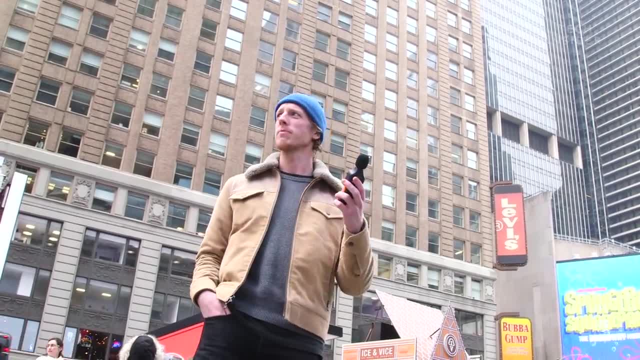 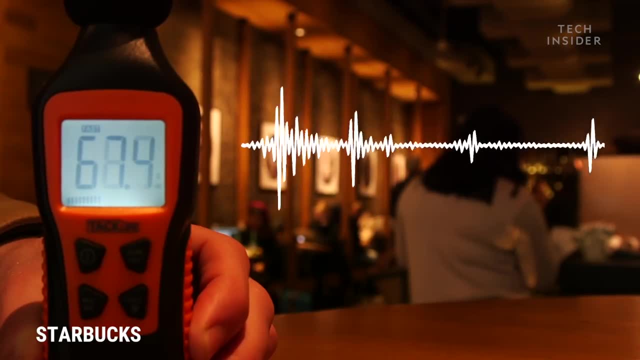 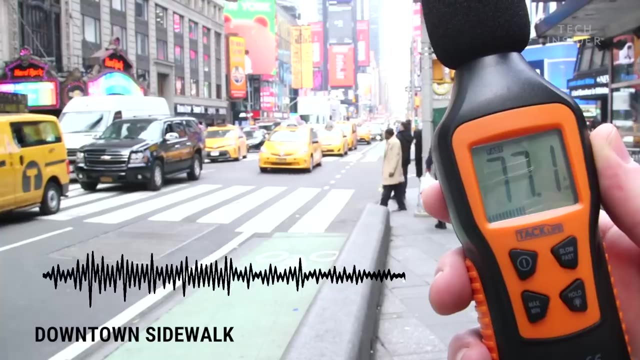 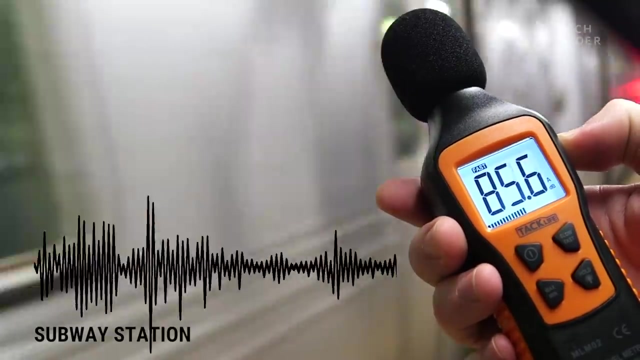 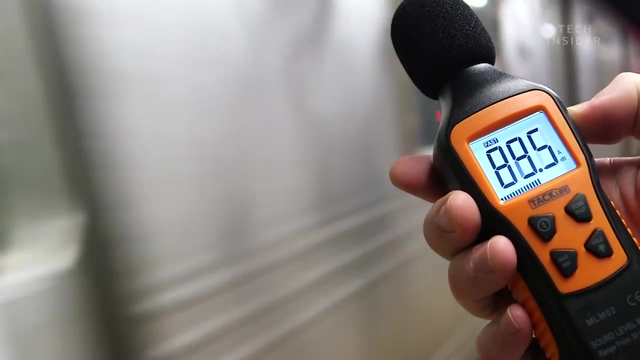 This is what an average New Yorker hears every day. Over time, we can get used to these sounds, but that doesn't make them any less dangerous. My name is Kit Frank. I am an audiologist. I work at NYU Langone. So I don't think we build up a tolerance to sound Anatomically. there's nothing that changes that can protect you from sound in your ear just because you're around it a lot. It's probably more of a psychological effect that you just don't notice it because you hear it all the time. In 2007,, researchers released results from their study on 200,000 hearing tests worldwide. They discovered that city residents had noticeable levels of hearing loss. Their hearing was what it should have been if they were 10 to 20 years older. 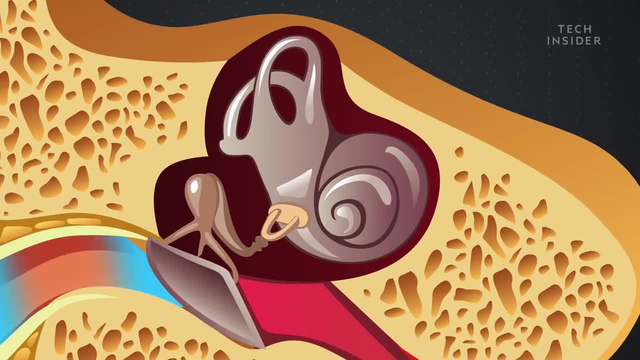 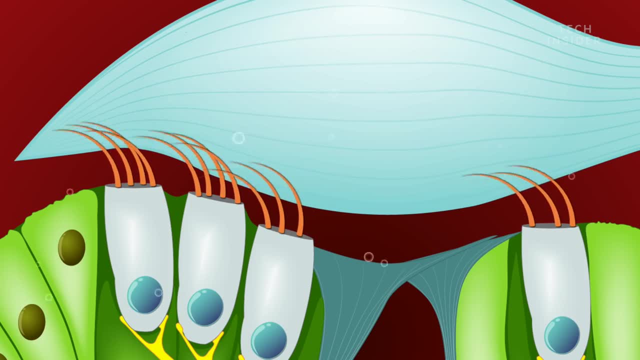 And once the damage is done, it's irreversible. We have microscopic hairs in our ears that relay sound to the brain. They're fine-tuned to detect vibrating frequencies from our eardrum. If those vibrations are too strong, it can bend, break or even destroy these delicate hairs. 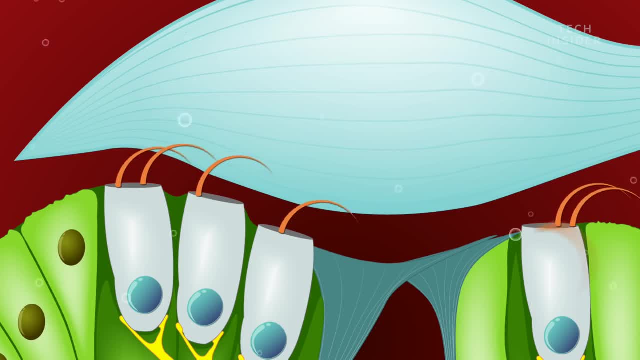 But unlike the hairs on your head, these don't grow back, Since we cannot see or feel these hairs. the damage from noise pollution is much less, But, unlike the hairs on your head, these don't grow back. If those vibrations are too strong, it can bend, break or even destroy these delicate hairs. 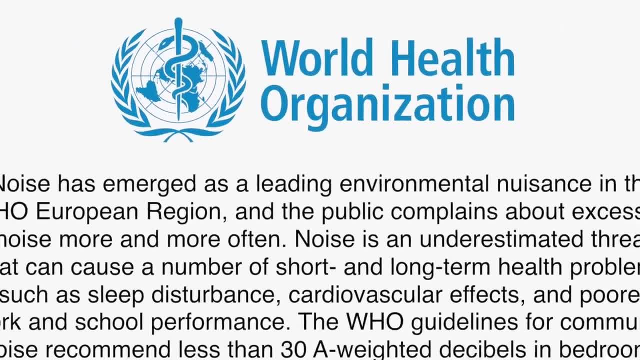 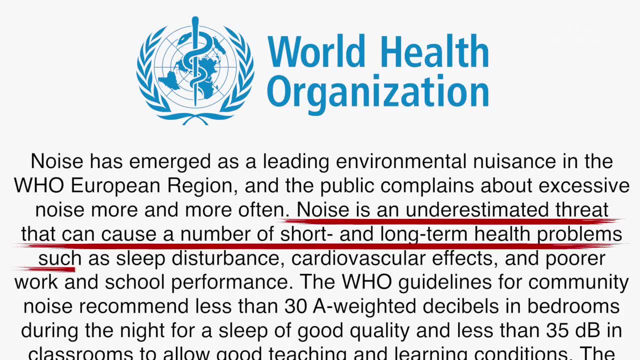 But unlike the hairs on your head, these don't grow back. According to the World Health Organization, noise is an underestimated threat that can cause a number of short and long-term health problems, such as sleep disturbance, cardiovascular effects and poorer work and school performance. 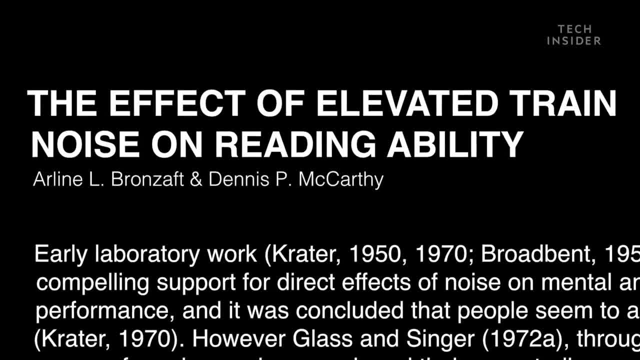 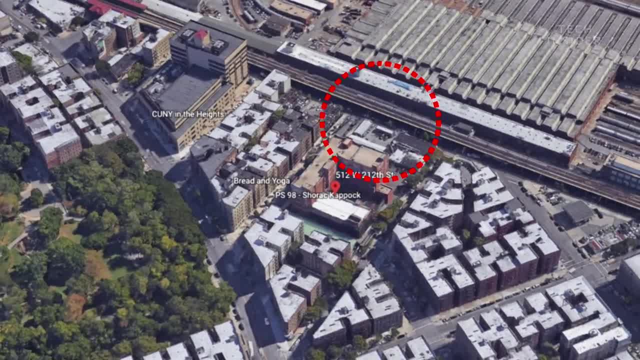 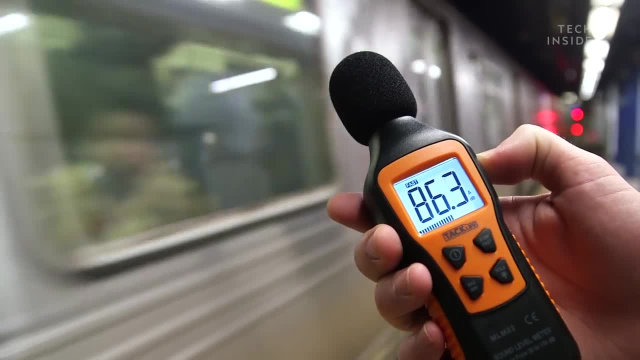 One of the most famous studies on noise pollution was in 1974. It happened here at Public School 98 in New York City. The east side of the building faces the subway. When trains passed, the noise pollution in the classroom went from an average of 59 decibels to 89.. 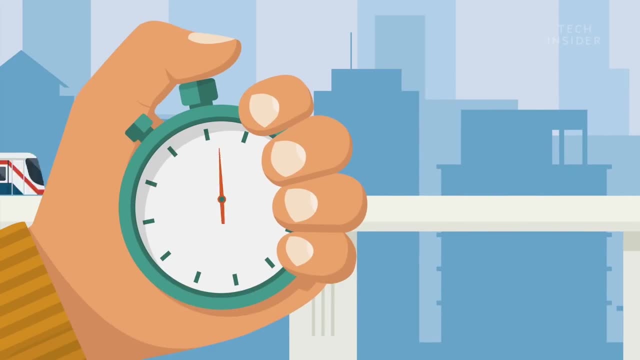 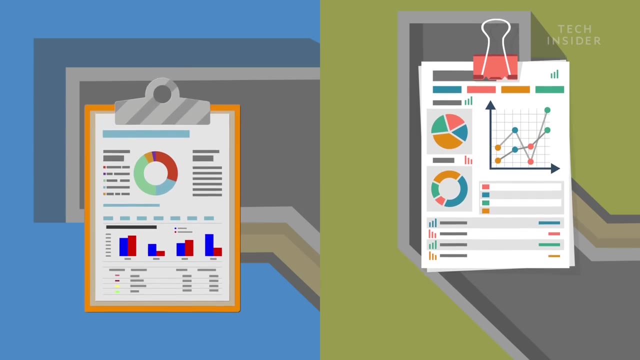 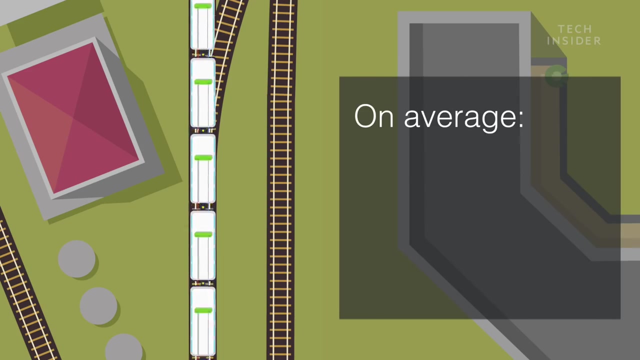 Teachers had to shout over the noise, And this happened about every four and a half minutes for 30 seconds at a time. The two researchers compared test scores and reading levels of students on the east versus the west sides of the building. While students on the west side weren't affected, students on the east side were, on average, four months behind on reading level. 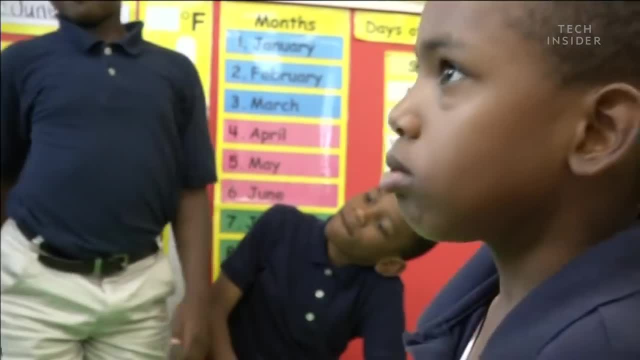 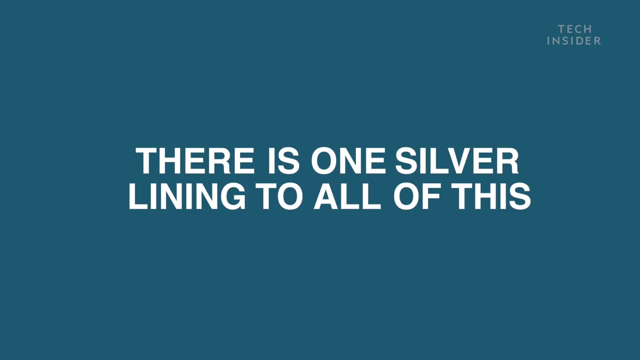 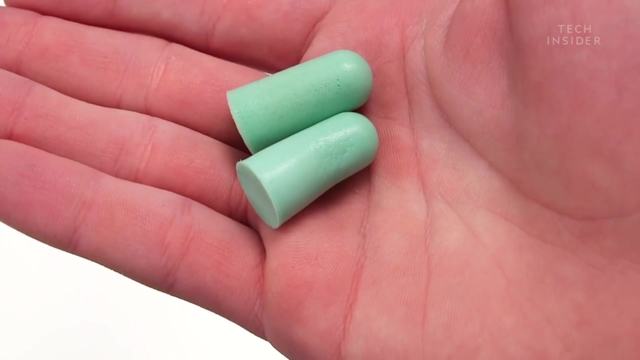 and they performed worse on achievement tests. More studies have gone on to show that children who live in noisy environments have elevated blood pressure and stress hormones. There is one silver lining to all of this: A pair of inexpensive earplugs are an easy temporary fix to this problem.